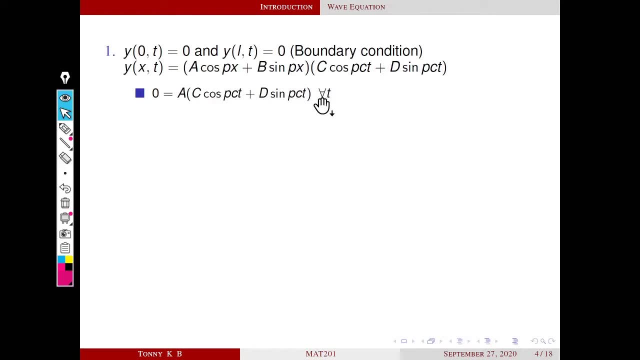 a times c, cos pct plus d, sin pct, for all t. As, similar to the previous cases, this term is non-zero. If this term is 0,, then this is 0. That means y is throughout 0. That means there is no displacement. 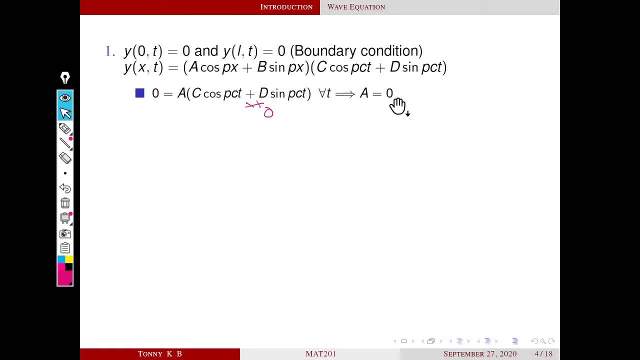 So this implies a should be 0.. Okay, Substitute a equal to 0 in this equation. Then we get y x t equal to b sin px into c cos pct plus d sin pct. If we multiply this b into the bracket, this time is bc and this time is bd. Here b and c are arbitrary. Okay, So 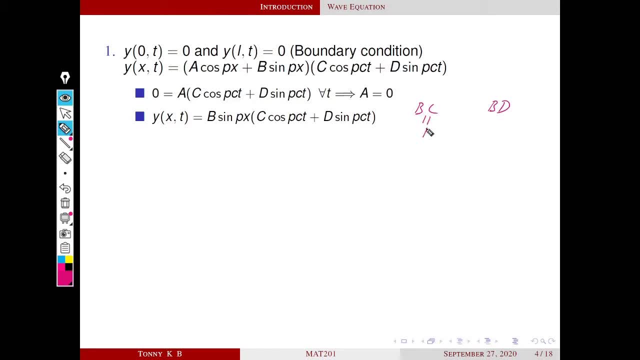 bc also arbitrary, So we denote that arbitrary by e. And similarly b and d are arbitrary, So bd is also an arbitrary. We denote it by f, So this expression become y, x, t equal to sin px. into this bc become e, So e, cos, pct plus. 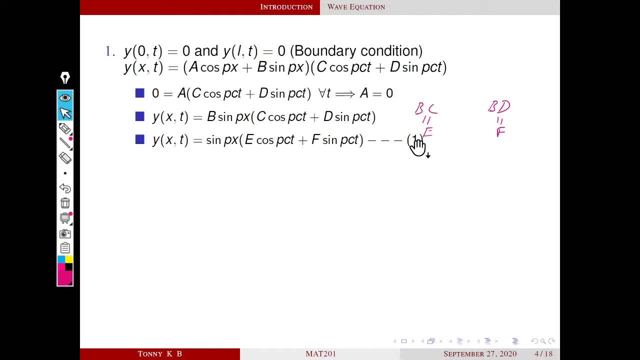 f sin pct. We denote this equation by 1.. Okay, Next we are going to apply the second boundary condition. We substitute x equal to l. When x equal to l, the left hand side become y, l, t. That is 0.. Okay, What about the right hand side? Right hand side is 0.. That means 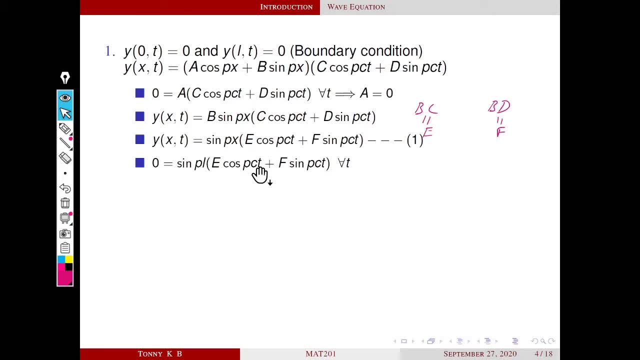 sin pl, So 0 equal to sin pl into e cos pct plus f sin pct for all t. As, similar to this case, this is non-zero. If this is 0, then our solution throughout 0. So this implies sin pl equal to 0.. Okay, Sin pl equal to 0 implies pl equal to n pi for all n belongs. 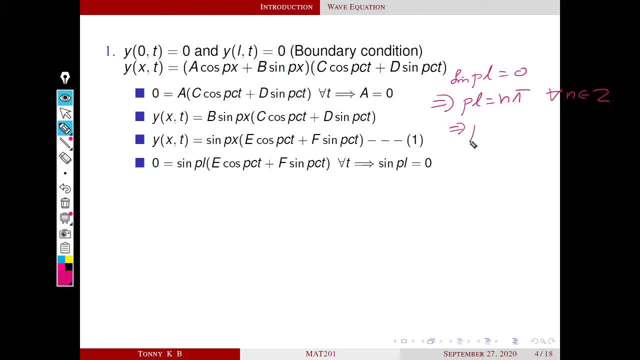 to z. That means set of all integers. So this implies So p equal to n pi by l, where n is an integer Substituting p equal to n pi by l in equation number 1, then we get pi x t equal to sin. 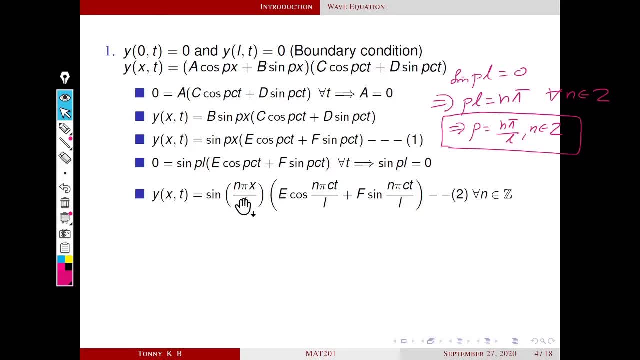 n pi x by l, because our p is n pi by l, e cos n pi ct by l, f sin n pi ct by l. This is true for every integer. So equation 2 is not a single solution. It is a collection of solutions. 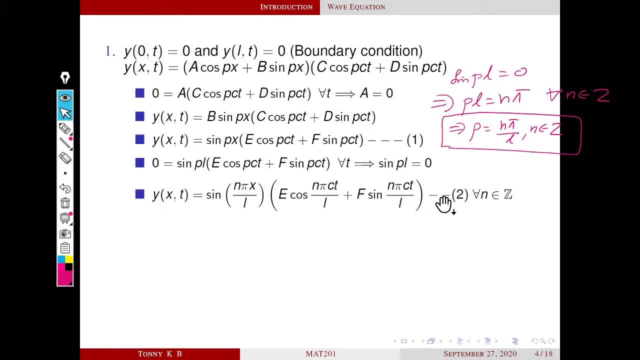 because whatever be the value of n, this gives a solution. Suppose n equal to 0. If n equal to 0, this becomes sin 0. Sin 0 is 0. So when n equal to 0, y, x, t become our trivial solution. 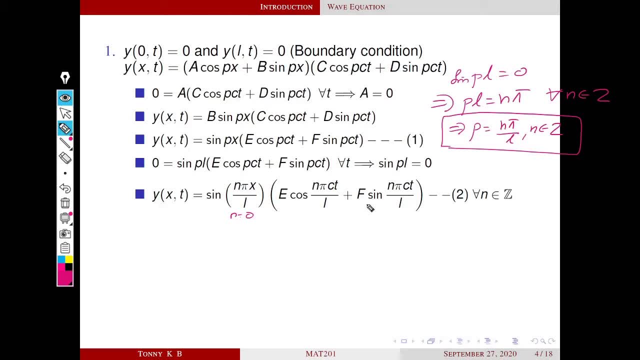 0 solution. Okay, we are interested only on non-zero solutions. So we throw out the case n equal to 0.. So these are the non-zero solutions for all integers except 0. Also, this arbitrary constants are different for each n. 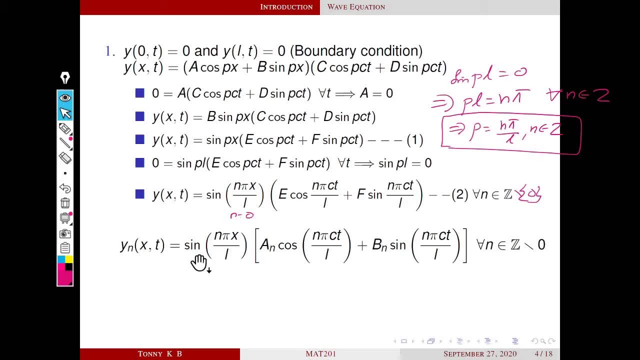 We rewrite this equation, number 2, as yn of xt is equal to sin n pi x by l into this an. So this arbitrary constant depends on n. So, replacing this e by an, an cos n pi ct by l plus and bn sin n pi ct by l, 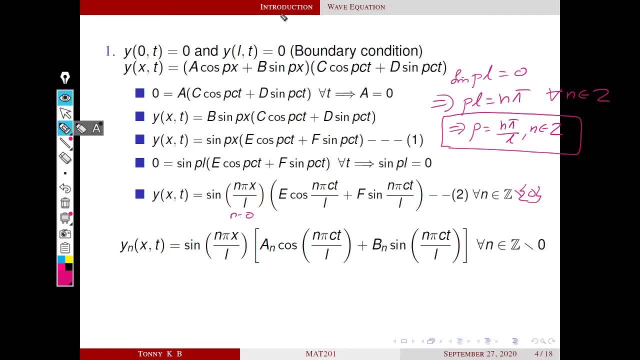 Okay, for all n belongs to z minus 0. One property of linear homogeneous equation is: if y1 and y2 are two solutions of a linear homogeneous equation, then their sum, y1 plus y2, is also a solution of linear homogeneous PDE. 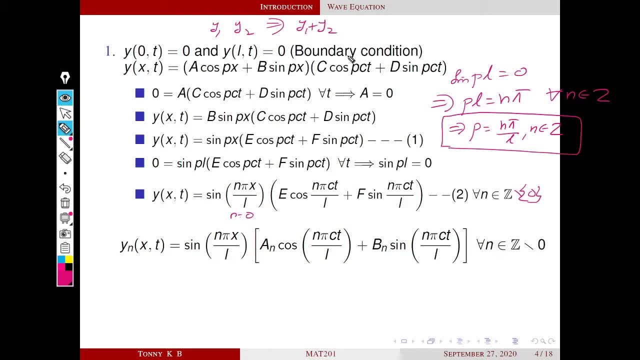 Okay, so our equation is a linear, homogeneous. So if yn's are solutions, so their infinite sum, their sum, is also a solution. This become yxt equal to. so most general solution, yxt equal to sigma n belongs to z minus 0. sin n pi x by l into an cos n pi ct by l plus bn. sin n pi ct by l. 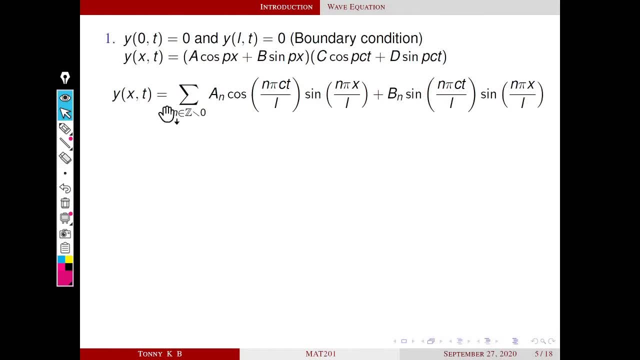 If you expand this bracket then we get yxt equal to, like this: Okay, another important thing is: suppose n equal to 1.. Suppose n equal to 1.. Then what is the term corresponding to n equal to 1?? And similarly, suppose n equal to minus 1.. 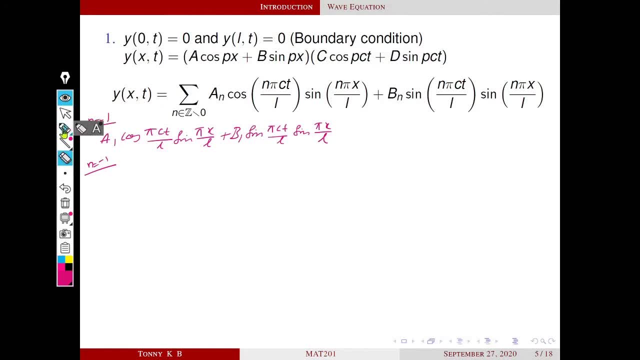 Then what is the term corresponding to minus 1?? This is equal to cos minus, theta is cos theta, So this become cos pi ct by l, similar to this term. This is sin minus theta form, that is, minus sin theta. Okay, so the first term is: 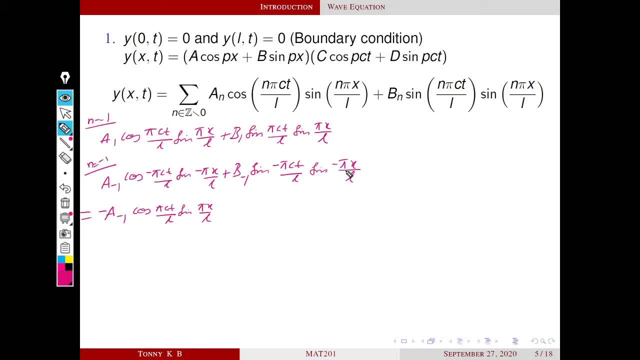 this is minus of sin. this is also minus of sin. So minus minus plus. So this become next we comparing these two terms: This is corresponding to n equal to 1.. This is corresponding to n equal to minus 1.. 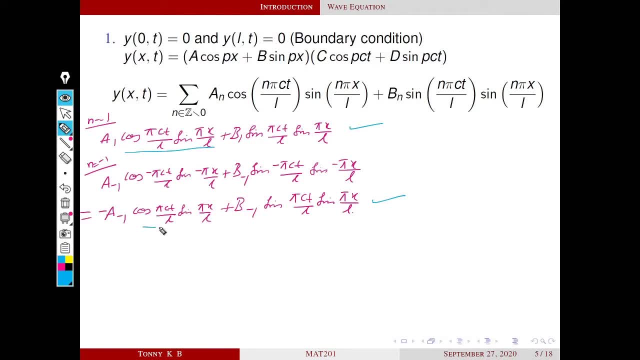 Okay, these two terms are same. Right, similarly, these two terms are same. You can, you can add the terms corresponding to n equal to 1 and n equal to minus 1.. Then, what happen Then? ultimately, then we get: 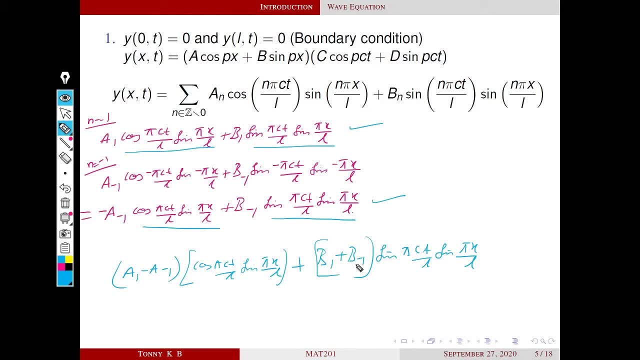 So this is the sum of the two terms corresponding to n equal to 1 and n equal to minus 1.. Okay, it is clear that here a1 and a minus 1, both are arbitrary. Okay, so we can replace this difference by another arbitrary, that is, a1.. 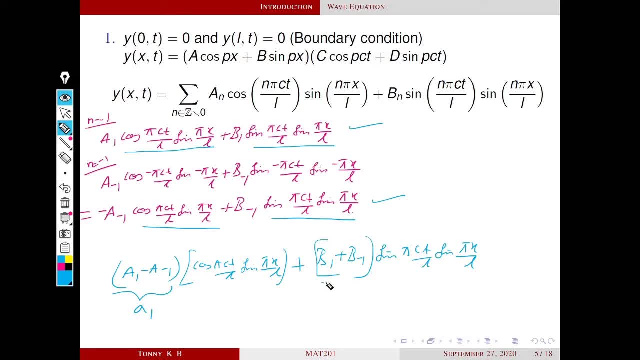 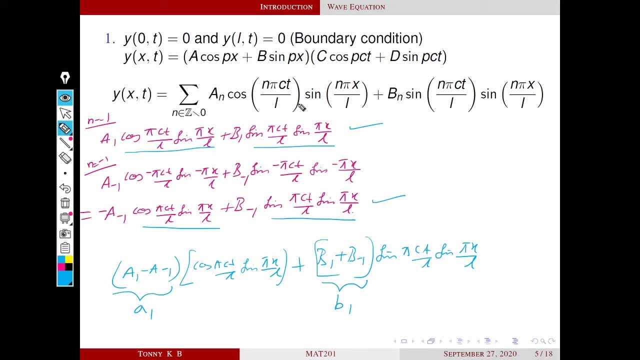 Similarly, if you compare the positive and negative corresponding terms, that means the terms corresponding to 2 and minus 2 and terms corresponding to 3 and minus 3, like that. Okay, then we get yxt equal to sigma, n, equal to 1 to infinity. 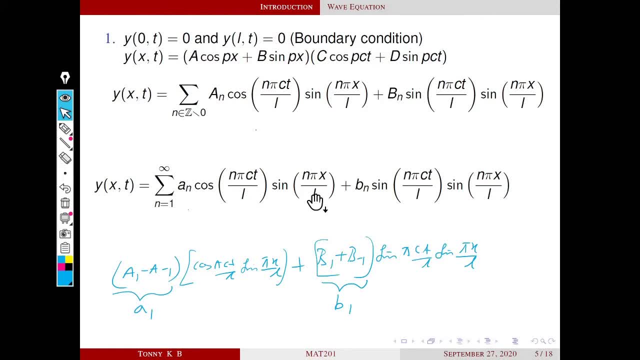 an cos n pi ct by l sin n pi x by l, plus bn sin n pi ct by l sin n pi x by l. Then, what is an and what is bn? What is an in terms of this capital an and capital bn, And similarly, what is bn? 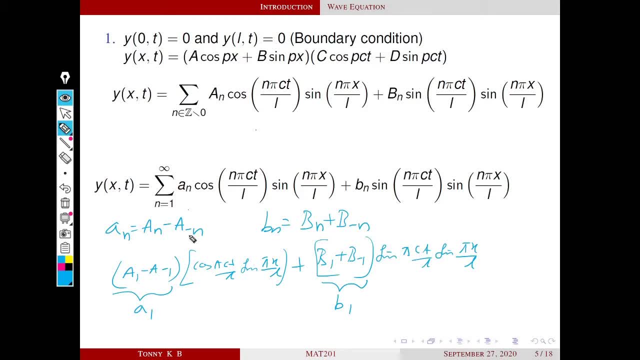 Here an and a minus n are arbitrary, So their difference is also arbitrary. That is replaced by small i. Similarly bn and this b minus n are arbitrary, So their sum is also arbitrary. So we are replacing that quantity by small bn. 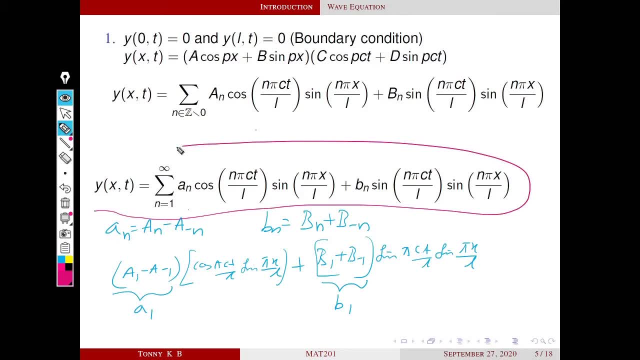 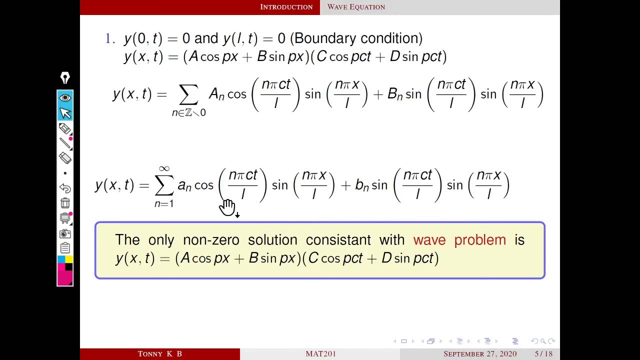 This is the non-zero solution derived from our third separable solution. This is the justification for the statement mentioned in the previous session. Okay, Here sin n, pi, x by l is common, So you can take outside. We can find this an and bn using initial conditions. 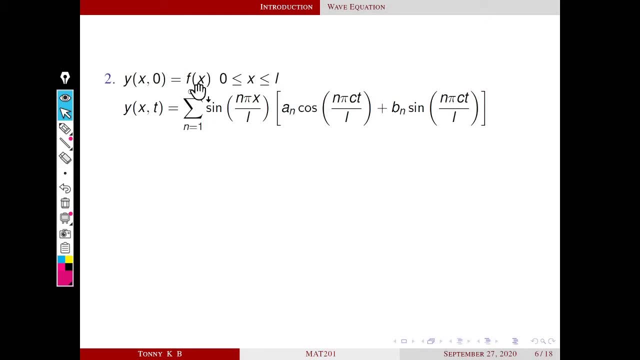 So first we are going to apply this initial condition, That is initial shape. We substitute t equal to 0. Then left side become yx0. And we know that yx0 is f of x When t equal to 0, this term is 1.. 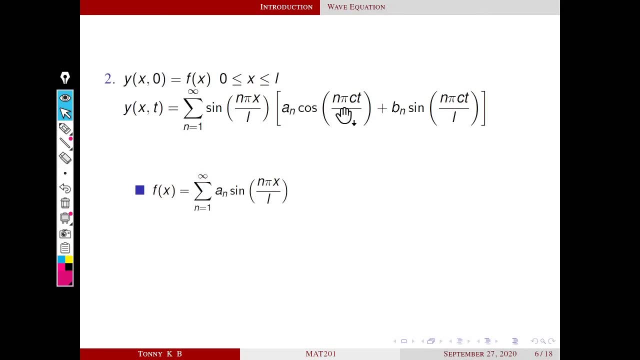 And this term is 0. Sin 0 is 0. So this expression become an. So this expression become an. So this infinite series become sigma an into sin n pi x. by l Right, This means f of x in terms of sin. 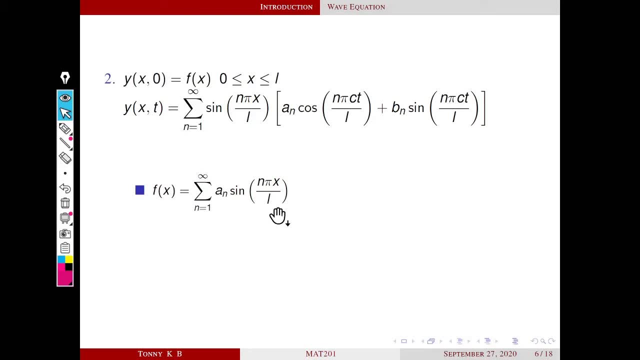 Are you familiar with such expression? Yes, This is the Fourier sin series of f of x in the interval 0 to l. So what is an? What is the Fourier coefficient? N is 2 by l, 0 to l. 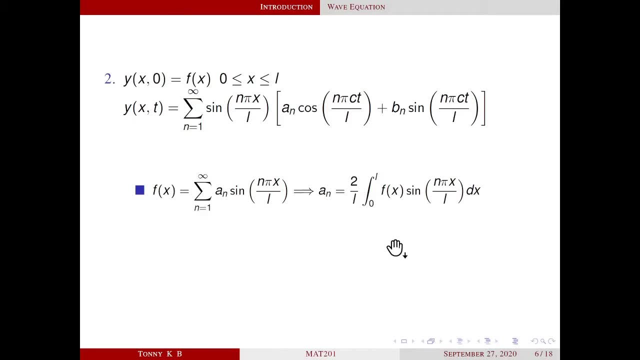 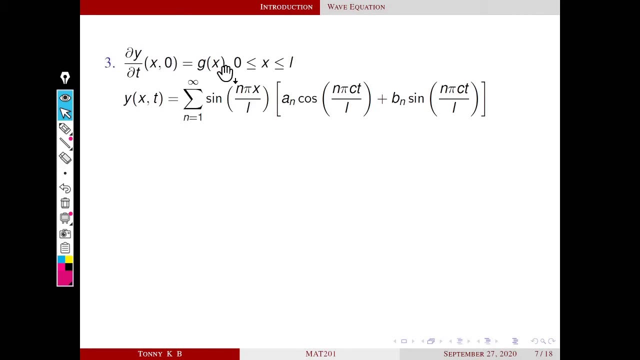 f of x sin n pi x by l tx. We have one more initial condition, That is, initial velocity. Partial dy by dt at t equal to 0 is g of x, So g of x is 0. Okay, So first we consider the derivative of our solution. 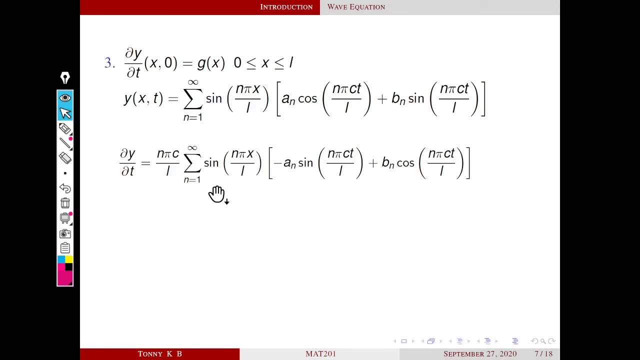 Okay, So this is the derivative with respect to t. Then you substitute t equal to 0.. So left, Left hand side become yx0.. Right hand side become g of x. What about the right hand side When t equal to 0, sin 0 is 0. 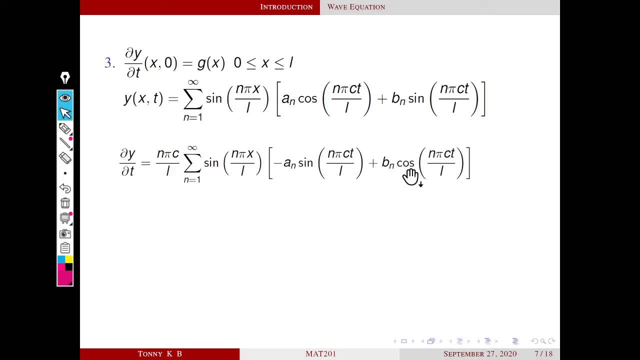 And this time is 1.. So cos is 1.. So this become bn. Okay, So when t equal to 0, this expression become g of x is equal to sigma, n equal to 1, to infinity bn times. n pi c by l into sin, n pi x by l. 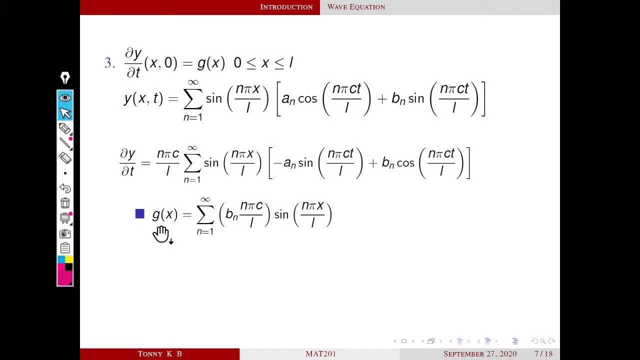 So this is the Fourier sin series of g of x, Right? So this bn into n pi c, bn into n pi c by l is the Fourier coefficient. Okay, So what about the Fourier coefficient Here? the Fourier coefficient is bn into n pi c by l. 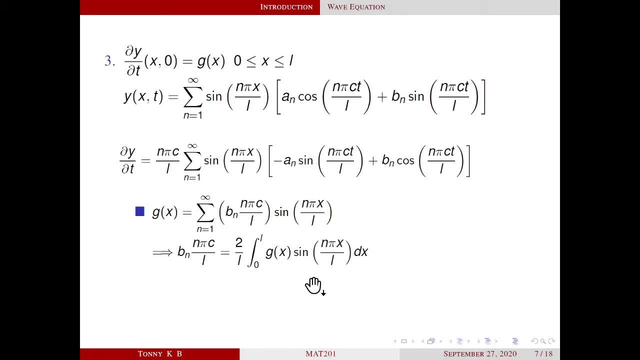 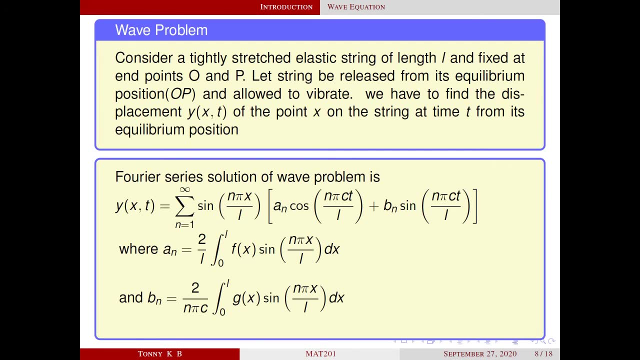 That is equal to 2 by l 0 to l g of x into sin n, pi x by l dx, And this implies bn is equal to: like this: Now the problem is completely solved. So this is the solution of our problem. 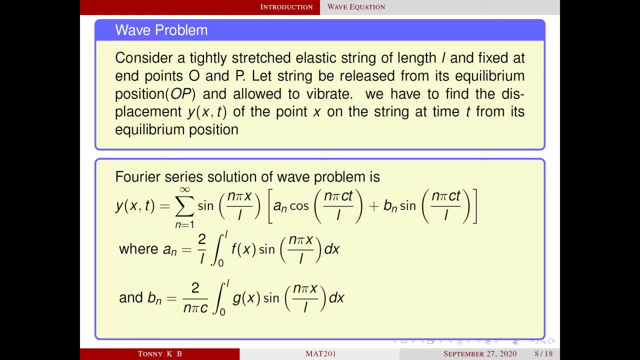 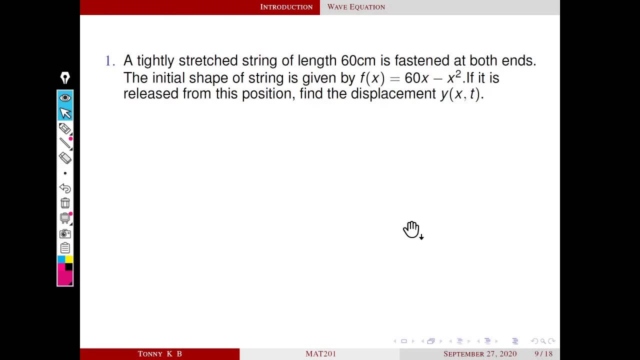 This solution is called Fourier series solution. Okay, So yx t equal to like this: Here a? n is given by a n and b? n are given by these formulas. Consider a problem: A tightly stretched string of length of 60 centimeter is fastened at both ends. 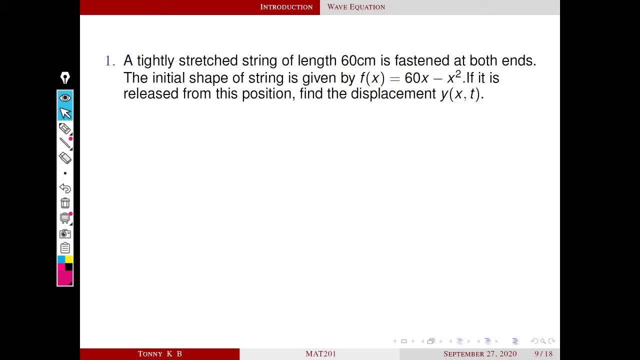 The initial shape of the string is given by f of x equal to 60 x minus x square. If it is released from this position, find the displacement yx t. Okay, So what are the given conditions? So the given conditions are: 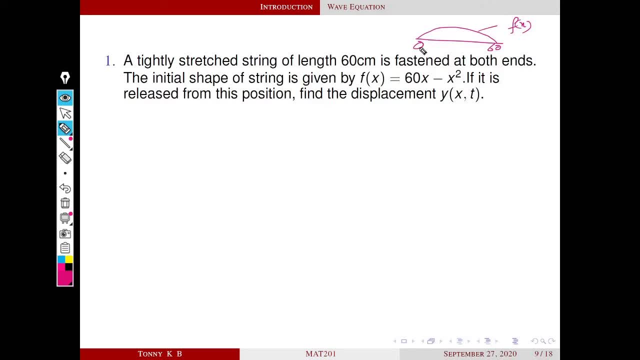 The length is 60.. So fixed at n point, So at 0 and 60.. So here our l is 60.. Right And initial shape of the string is given, So f of x is given. That is 60 x minus x square. 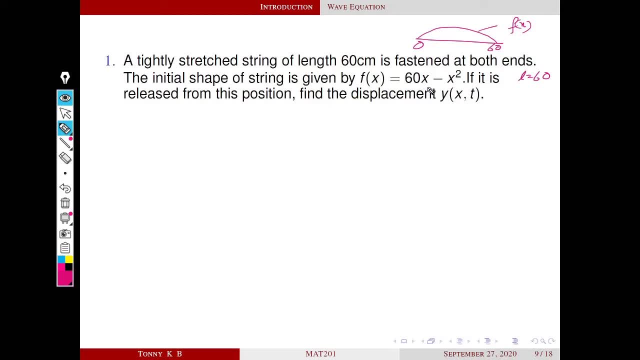 And it is released from this position Just released. So what about the initial velocity? Yes, it is 0. That means g of x is given, That is equal to 0.. These are the given conditions: y 0, t equal to 0 and y 60 t. 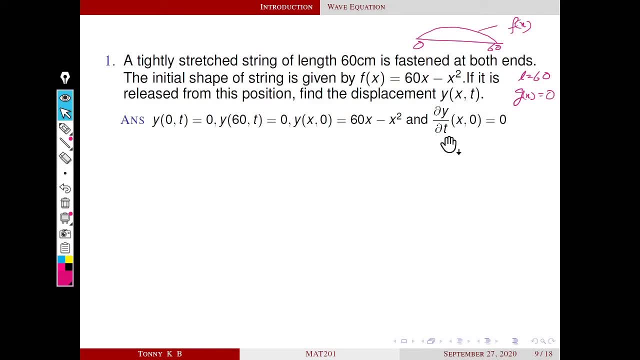 And initial shape is 60 x minus x square, And initial velocity is 0.. And we know that this is the general solution of the work problem. We are simply replacing l by 60.. Okay, And you can easily find a? n and b? n using our Fourier coefficients. 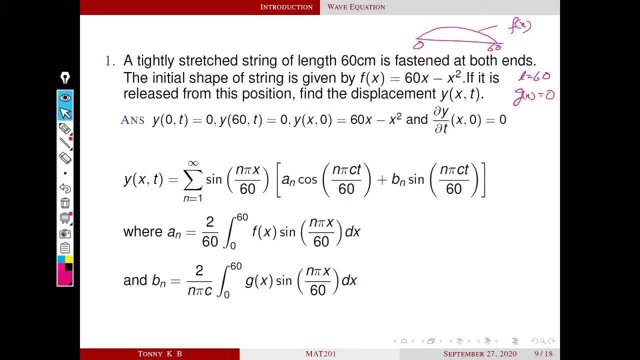 So what is a n? You can evaluate a n using this formula, Replacing l by 60. And similarly b n's by this formula. So here, g of x is 0.. Initial velocity is 0.. So what about this integral? 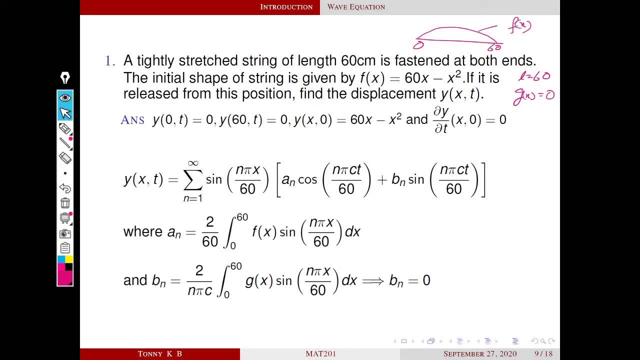 Whatever the value of n, this integral is always 0.. This implies all the b n's are 0.. Next we have to find a n's By substituting f of x as 60 x minus x square 1 by 30 integrals 0 to 60.. 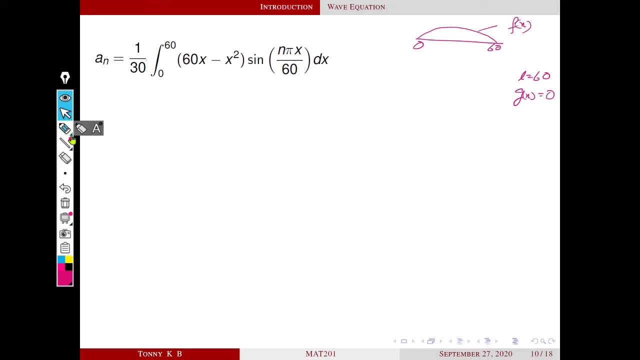 60 x minus x square into sine n pi x by 60 dx. Next, we are going to integrate this using general rule of integration By parts, That is, integral u v x is equal to u into integral of v 1. We denote lower suffix for integration, upper suffix for derivative. 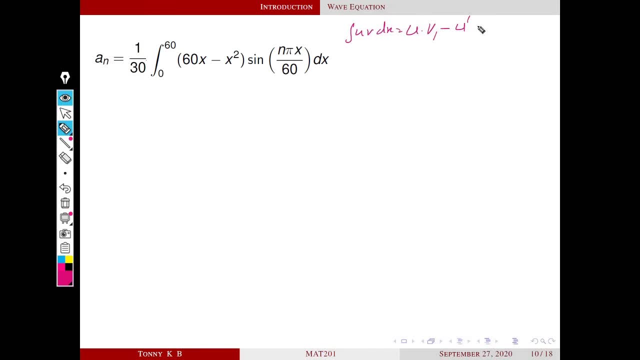 Minus u 1.. So u 1 stands for derivative of u v 2.. So what is v 2?? v 2 is the integral of v 1.. Okay, And plus u 2, v 3 minus plus, etc. 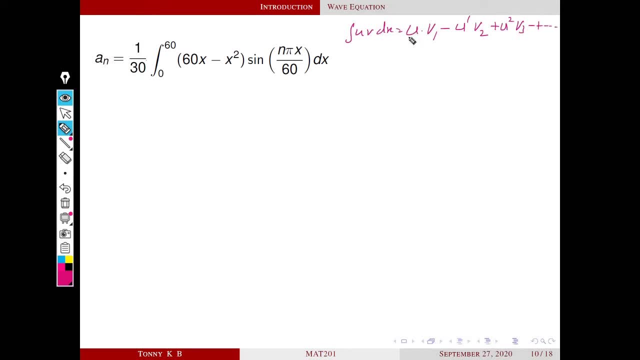 And this formula is applicable only when The derivative of first term should 0 after final number of steps. Okay, So applying this formula to this equation Here, we are treating this as our u, This as our v, So this become 1 by 30.. 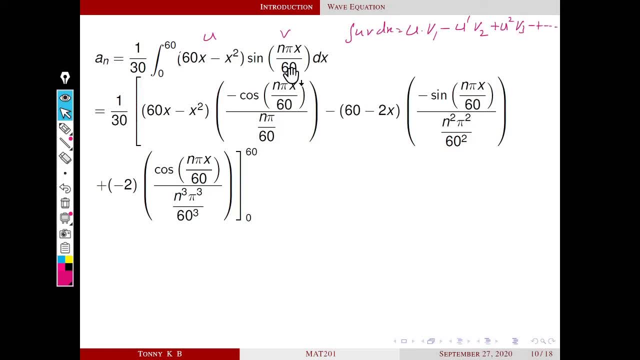 Yes, u is 60 x minus x square And u into v 1. v 1 means integral of v. So what is integral of sine? That is minus cos n pi x by 60. Divided by n pi by 60.. 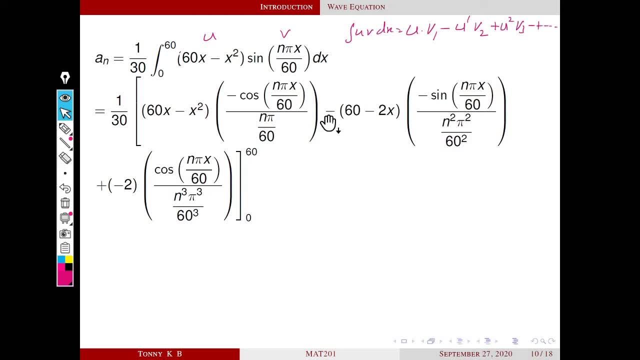 Okay, Then minus u dash. This is our minus sign, u dash, Derivative of this expression. That is 60 minus 2 x. Right Then v 2.. What is v 2? v 2 is, You should remember, v 2 is integral of v 1.. 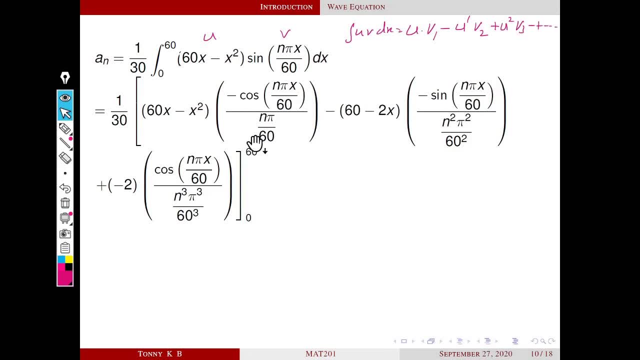 This is our v 1.. This entire thing, Including this minus. Okay, This is our v 1.. So what is the integral of v 1?? The integral of cos is sine. There is a one minus sine. So minus sine n pi x by 60.. 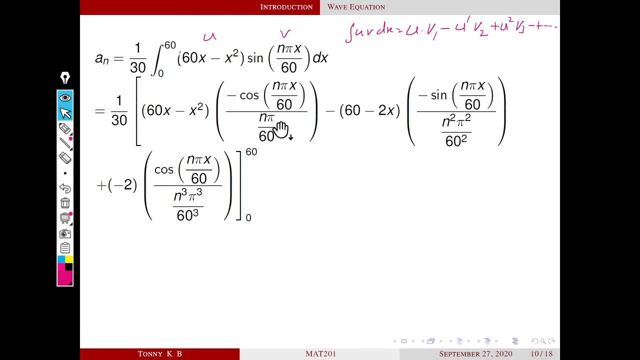 Divided by n pi x by 60.. Already, one n pi x by 60 is here. That is why this is n square pi square by 60 square. And what about the third term? Third term is plus, Yes, plus. 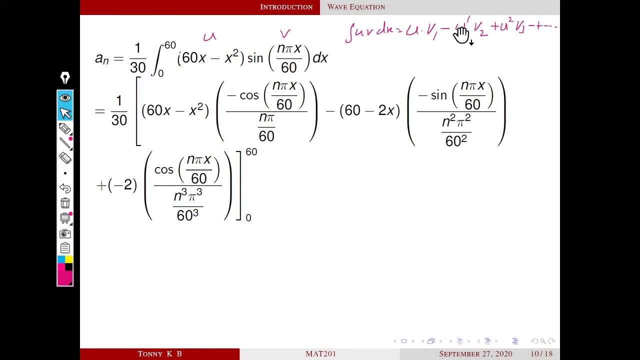 u 2.. u 2 means second derivative of u Or derivative of u 1. This is our u 1.. Okay, So what is the derivative of 60 minus 2? x? That is minus 2.. And v 3.. 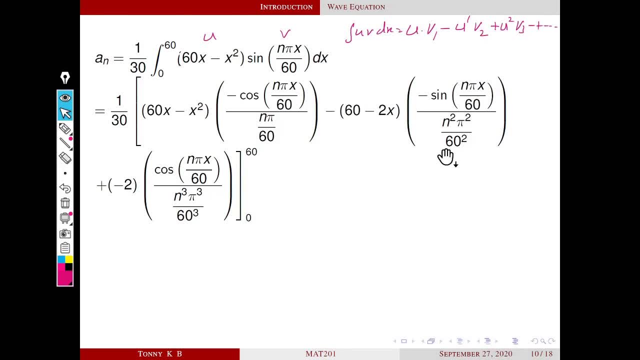 What is v 3?? v 3 is the integral of v 2.. This is our v 2. Right. Including this minus This Full Quantity is our v 2.. Okay, So integrate this v 2.. 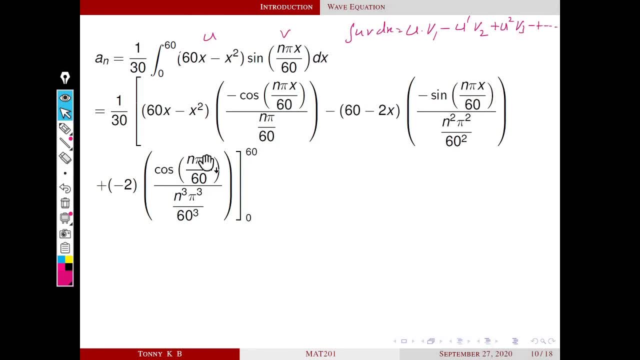 So that is again. integral of sine is minus cos. So minus minus, this become plus. That is why this is cos n pi x by 60, by n cube, pi cube by 60.. Okay, Then lower limit is 0.. 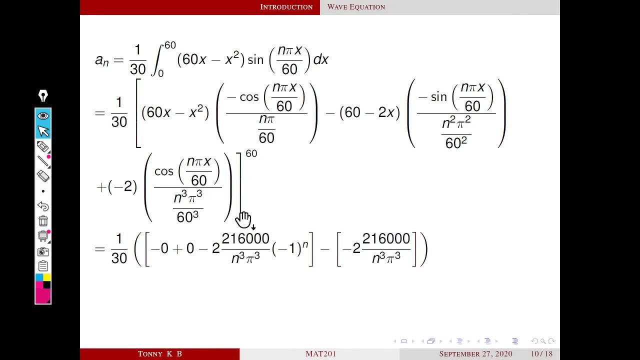 Upper limit is 60.. If you substitute upper limit and lower limit, Then we get like this, Because when x equal to 60.. This is 60 square minus 60 square, So this is 0.. And in second term, 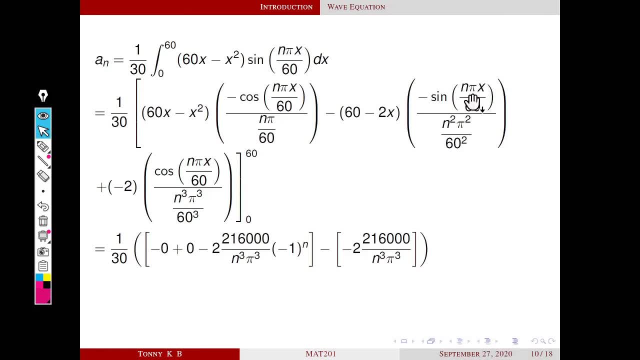 When x equal to 60. This becomes sine n Pi and sine n pi is 0.. Okay, And the last time is minus 2.. Yeah, minus 2.. It's reciprocal, is this one? And this become cos n pi, and cos n pi is minus 1 raised to n. 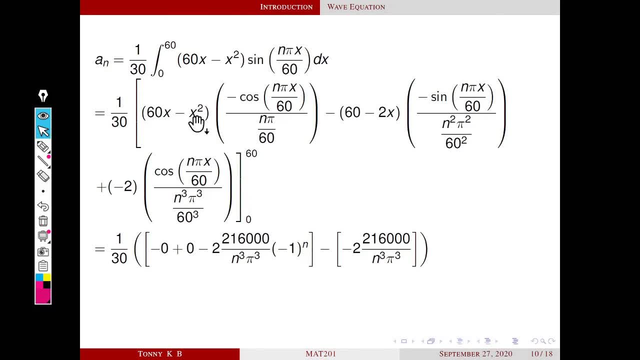 Minus. Then we substitute lower limit: 0.. When x equal to 0. This expression is 0 and here sine 0. So this one also 0.. When x equal to 0. This is 1.. So minus 2 times its reciprocal. 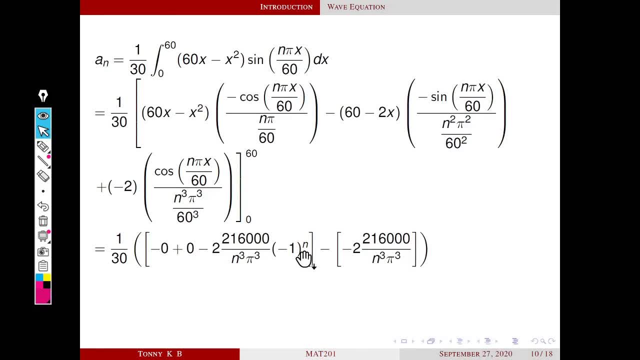 That is, 216 triple 0 by n cube pi. Okay, by simplifying this we get 1 4 4 0, 0 by n cube pi. cube into 1 minus minus 1 raised to n. This term become 1 and 1 minus minus 1 raised to n. 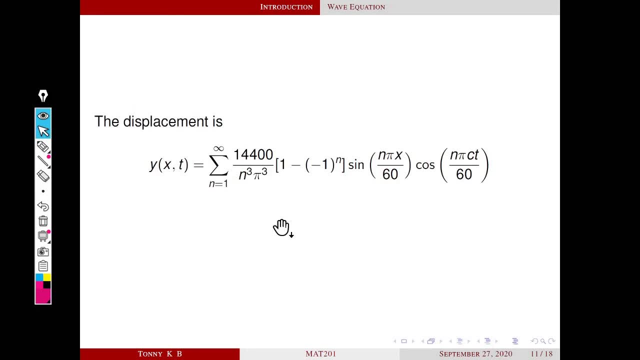 So this is our an. So the displacement function yxt is sigma n equal to 1 to infinity. This is our an an into sine n pi x by 60, cos n pi ct by 60. So this is the solution of our problem. 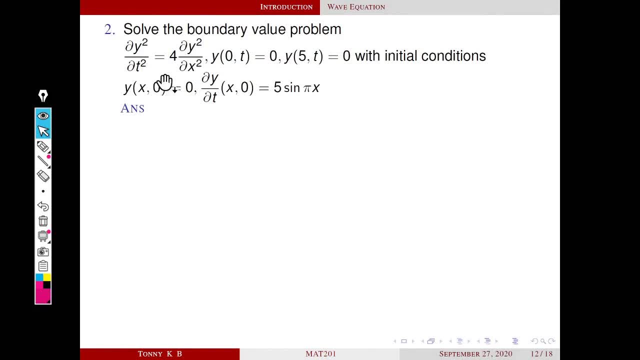 Next problem: solve the boundary value problem. partial dy square by dt square equal to 4 times partial dy square by dx square. This is our wave equation and with these two boundary conditions and two initial conditions, Okay. so here c square is given, here c square is 4, which implies we can take c as 2.. 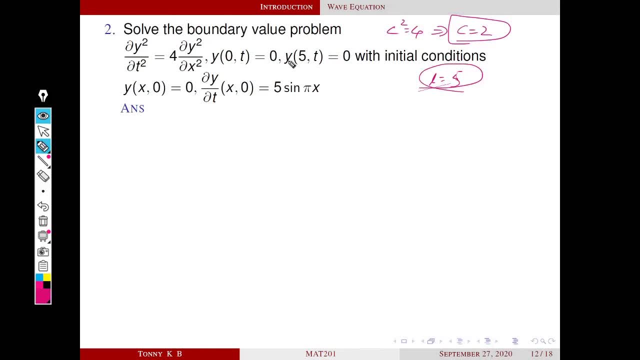 Here l is 5 because y 5t is 0. That means l equal to 5.. And what is f of x? Here, f of x is 0, because y x 0 is our f of x. What about this? 5 sine pi x? 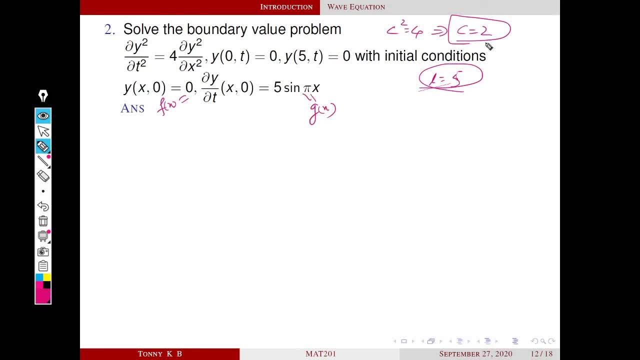 This is our g of x. So now everything is not: c is 2, l equal to 5, f of x is 0, g of x is 5 sine pi x. So we know that this is the solution of this problem. 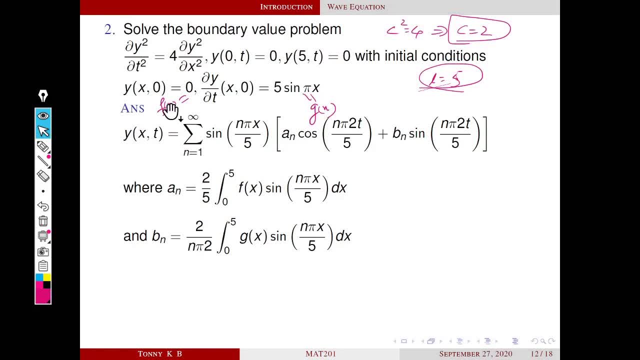 And replacing c by 2 and l by 5. So here f of x equal to 0.. So here l equal to 5.. a n's are 0.. You complete this problem. Either you can evaluate this integral by substituting g of x equal to sine pi x. 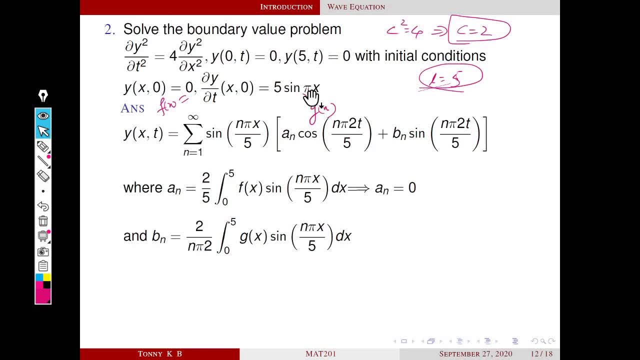 Otherwise, here the g of x is of the form sine pi x. From our previous discussion we know that this is the partial derivative. Then you substitute t equal to 0. So this become right side, become b n n pi 2 by 5 sine n pi x by 5..